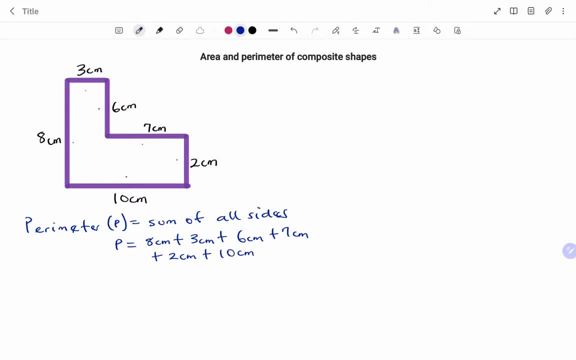 and plus 10 centimeters. Note that all the sides are counted for. Therefore, putting this in your calculator, you're going to have the perimeter equals to 36 centimeters To find the area of the shape, because it's a composite shape. 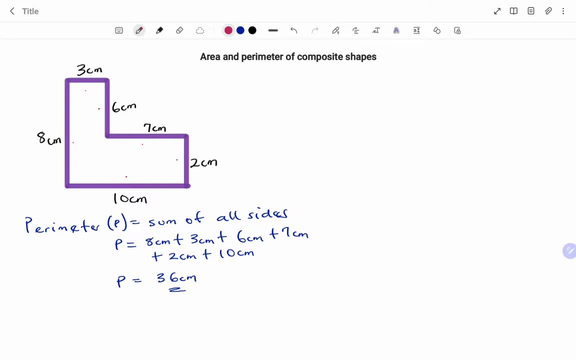 we need to divide the shape into two or more basic shapes. In this example, I'm going to divide the composite shape into two basic shapes. I have two rectangles, shape A and shape B, such that the area of the shape will be the area of shape A plus the area of shape B. 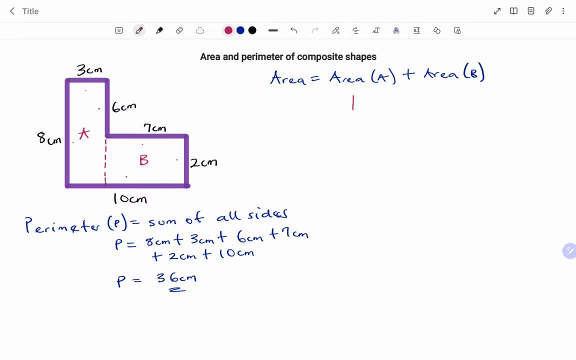 I'm going to draw a rough sketch of the shapes I have. shape A, a rectangle with sides eight centimeters and width three centimeters. The length is eight and the width is three. Shape B: I have it this way: The width is two centimeters and the length seven centimeters. 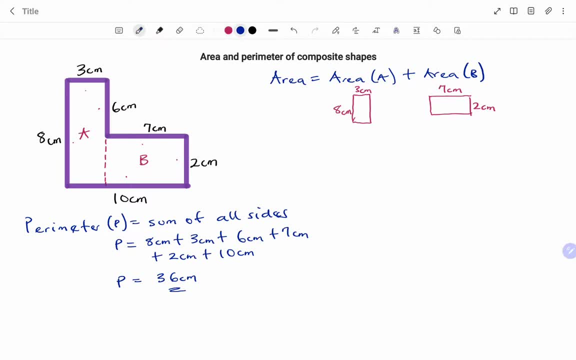 Using the formula for the area of a rectangle, which is the length times the width, I have L times the width, the length times the width. In this case, for shape A, the length is eight centimeters, So I'm going to multiply the length times the width, three centimeters plus the area. 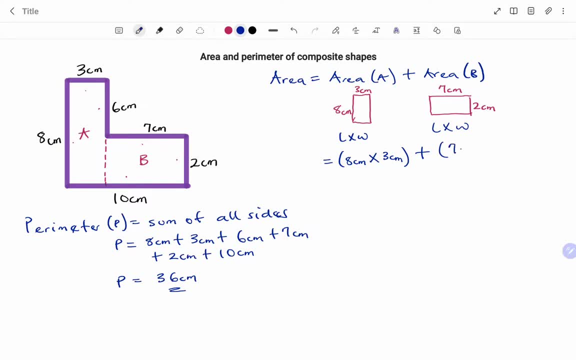 of the second shape, which has length, seven centimeters. So I'm going to multiply the length- seven centimeters- and width, two centimeters. Eight times three, that's 24 square centimeters, plus seven times two, that's 14 square centimeters. Adding it together, the total area is: 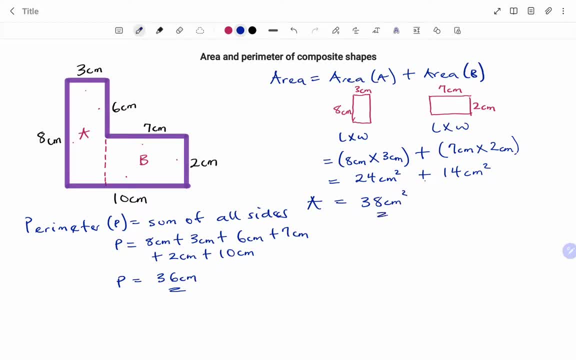 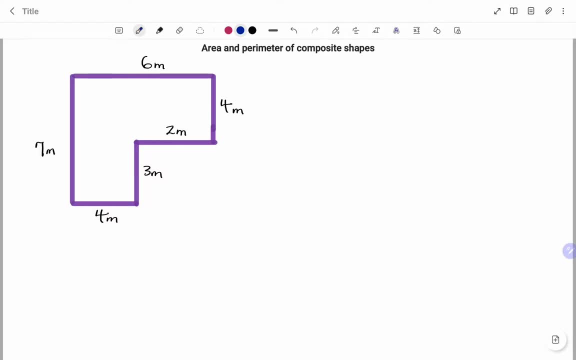 38 square centimeters. Let's look at another example. In the second example I have another composite shape with all the sides given. So find the perimeter. We need to add all the sides, So parameter equals sum of all sides. that's equal to seven meters plus six meters plus four meters plus two meters. 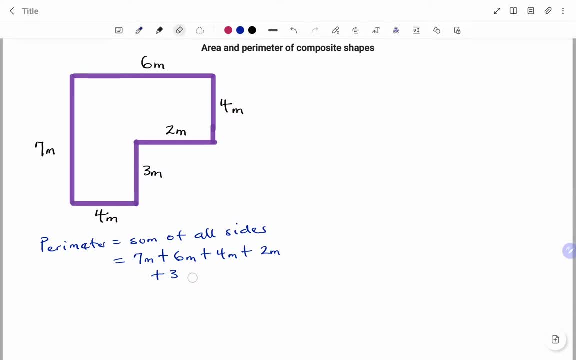 plus three meters again. That's going to change it to meters and 4 meters. Like I said earlier, you need to make sure that all the sides are counted for. So I have 1,, 2,, 3,, 4,, 5, 6 sides. 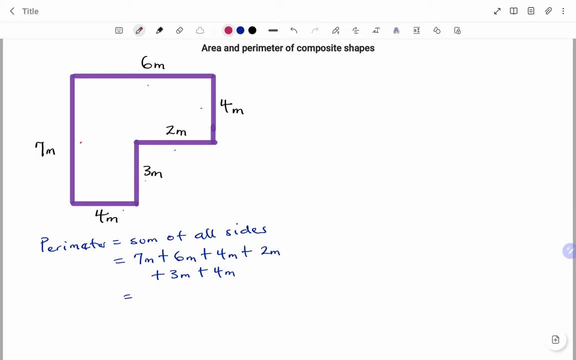 I have 7,, 6,, 4,, 2,, 3, and 4.. If I add that together, I'm going to have 26 meters as my perimeter To find the area. the area, because it's a composite shape. 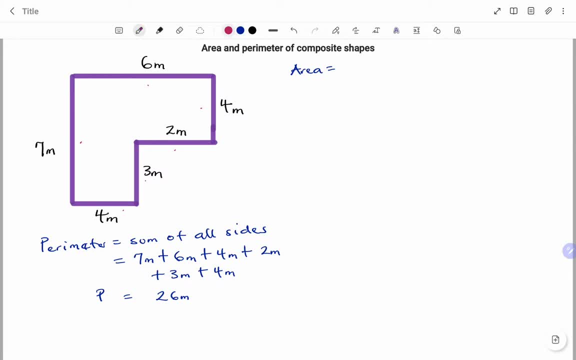 I'm going to split up the shape into basic shapes. If I cut my shape on this side, I have two shapes. I have shape A and shape B, So the total area will be area of shape A plus area of shape B. I'm going to draw a rough sketch. 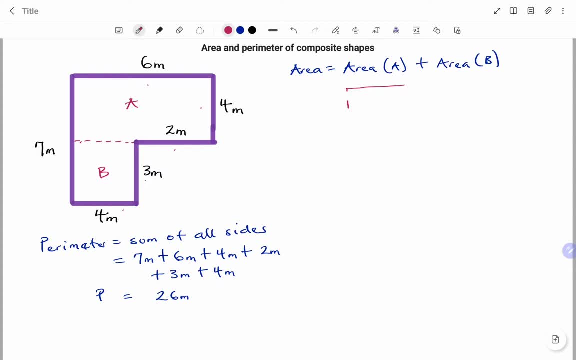 For the rough sketch of each shape, I have a rectangle with the dimension 6 meters and a width 4 meters. For the second shape, I have a smaller rectangle with length 4 meters and width 3 meters, Using the formula for a rectangle. 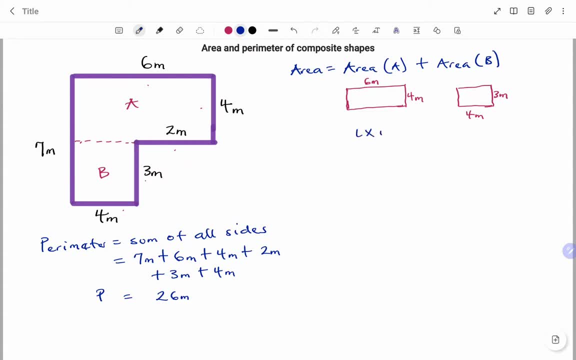 the area of a rectangle is. I have my length times my width, length times my width. Therefore, the area of this shape will be the area of the first triangle, that's A triangle B, that will be 6 meters times 4 meters. 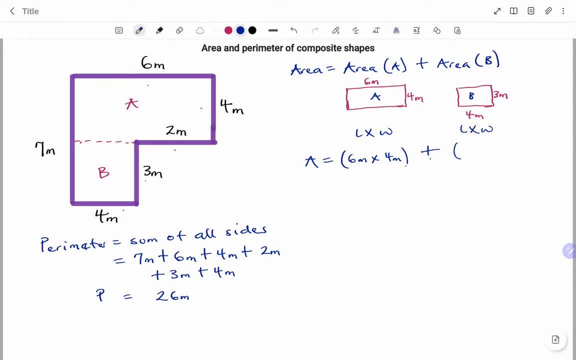 plus the area of the second rectangle, that's 3 meters times 4 meters, 6 times 4, that's 24 square meters plus 3 times 4, 12 square meters. Adding them together, the total area is 36 square meters. Thanks for watching, Bye.